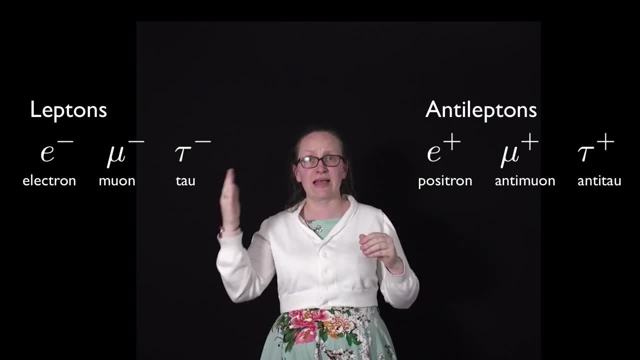 Now it turns out that each of these leptons and anti-leptons has an associated neutrino. So we've got an electron neutrino, a muon neutrino, a tau neutrino, as well as an anti-electron neutrino, an anti-muon neutrino and an anti-tau neutrino necesita. The neutrino does not force the reaction of the muons into truly cela. So leptons also. Saturday's Above刚rie takes advantage of any substance pressure in the particle sequence. So all the electrons in leptons exist in ourulletroょ. is any electron from one natron to a muon neutronкрinoойти. 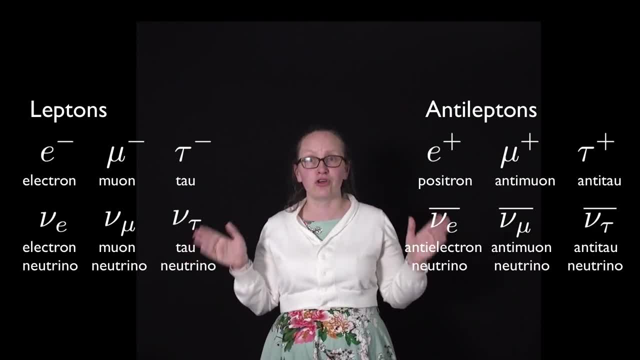 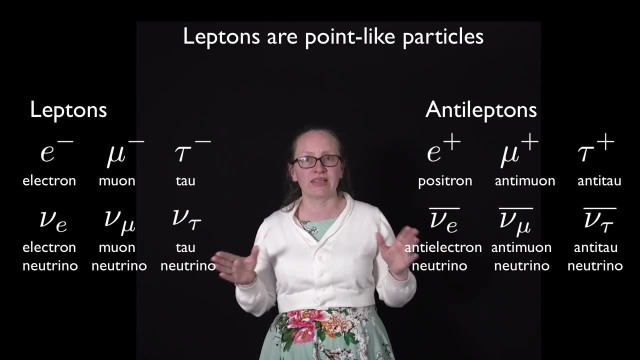 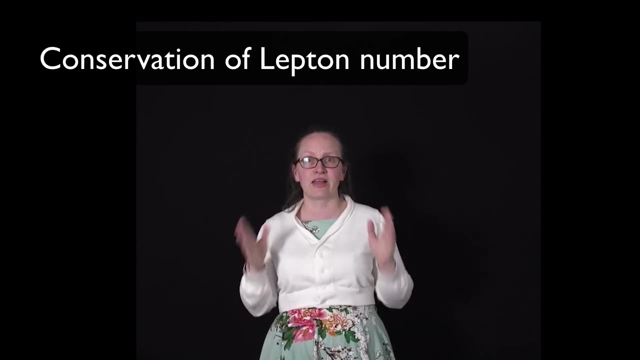 Neutrinos all have very, very low mass and no charge. All of our leptons have no internal structure or volume. They're essentially point-like particles. Now it turns out that leptons have their very own conservation law. We can consider the lepton number which. 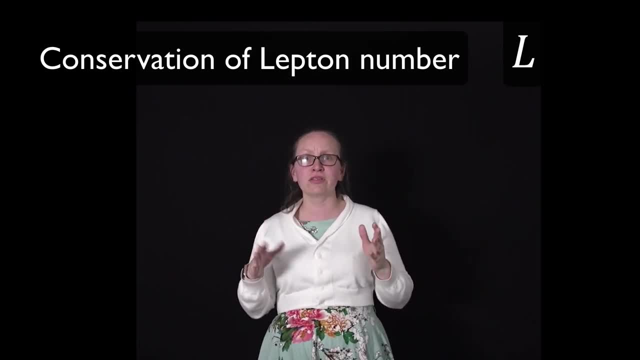 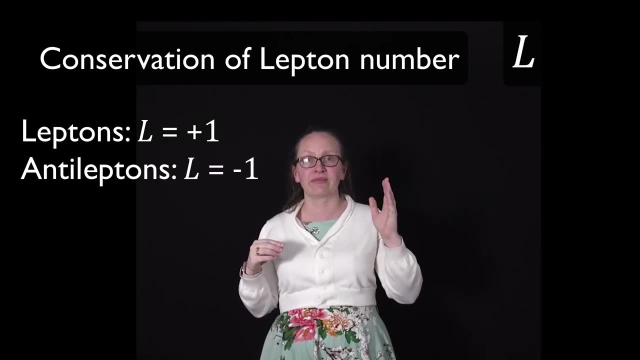 is given the symbol capital L For leptons. they all have a lepton number equal to plus 1, while anti-leptons all have a lepton number equal to minus 1.. Any particle which is not a lepton has a lepton number equal to 0.. 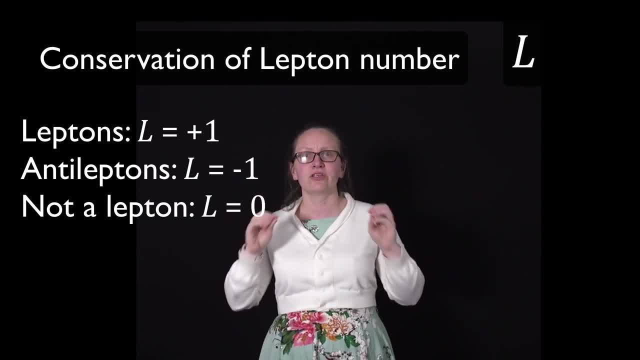 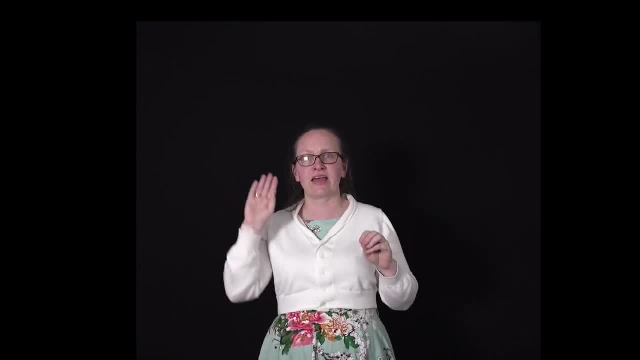 So let's use this lepton number conservation to consider a reaction we've already considered. We've considered the beta decay of a neutron. So we've seen that a neutron can decay into a proton, an electron, and we said that there must also. 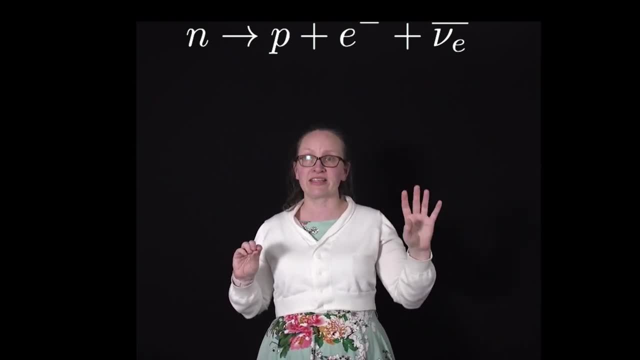 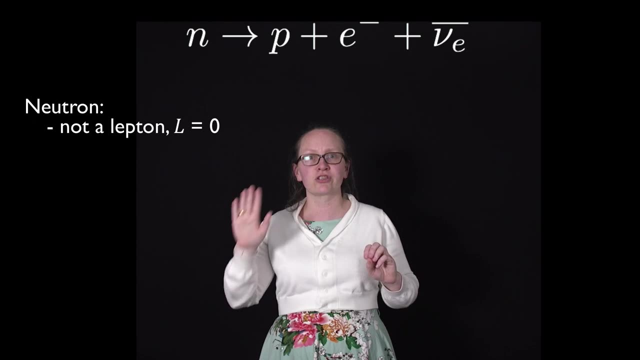 be an anti-electron neutrino. So we'll see why that is now So. on the left-hand side we've got a neutron. A neutron experiences a strong nuclear force, so it's not a lepton, so it has a lepton number of 0.. 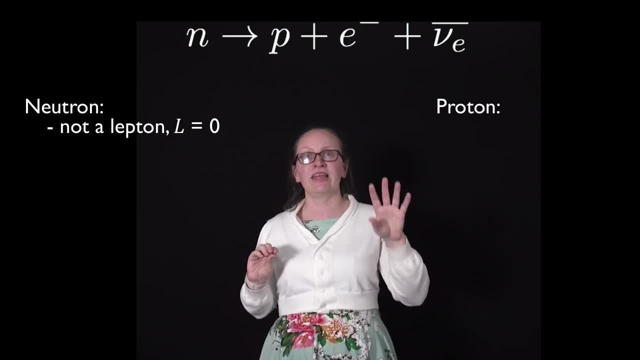 On the right-hand side, we've got our proton, which similarly has a lepton number equal to 0. We've also got the electron, which is a lepton, and so its lepton number is equal to plus 1.. And then the anti-electron neutrino. 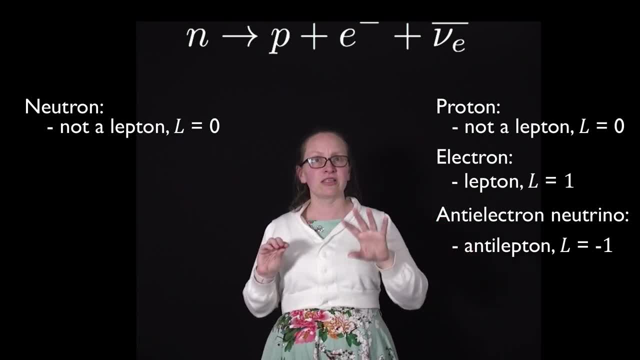 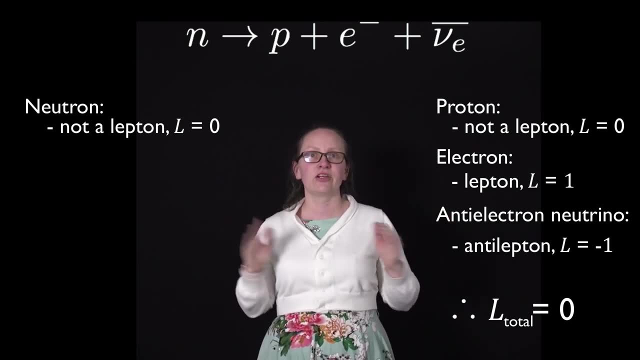 has a lepton number equal to negative 1.. So you can see, on the right-hand side we've got a total lepton number equal to plus 1, and then the to zero, which is equal to what we had on the left hand side. So this is part of 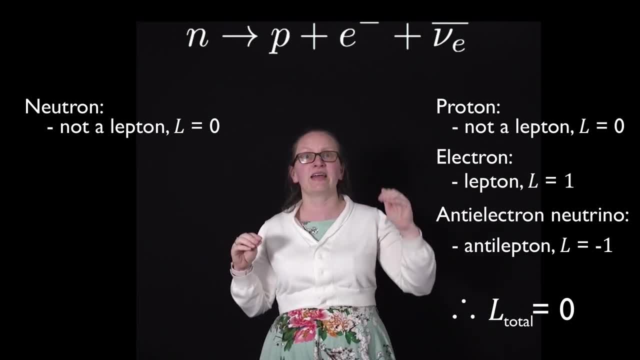 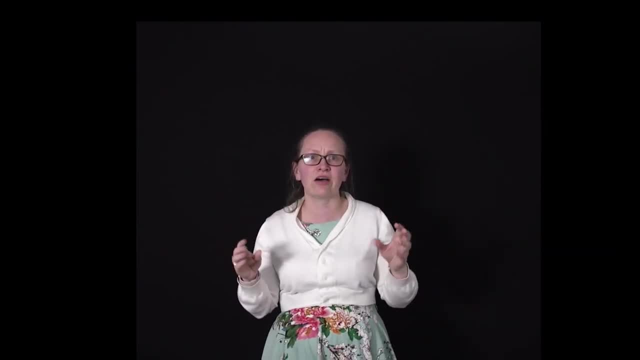 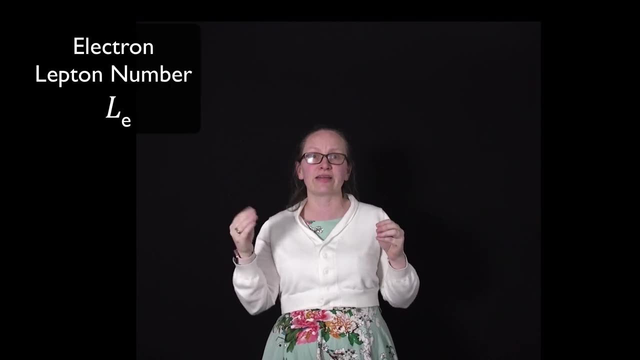 the reason why in a beta decay we get the anti electron neutrino formed as well as the electron. Now it turns out that we also have in most situations we have the conservation of electron. lepton number, muon lepton number and tau lepton. 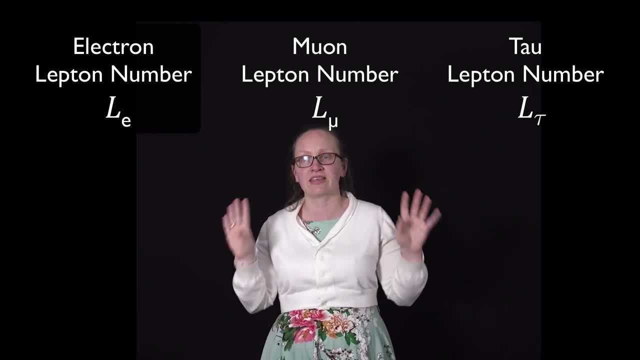 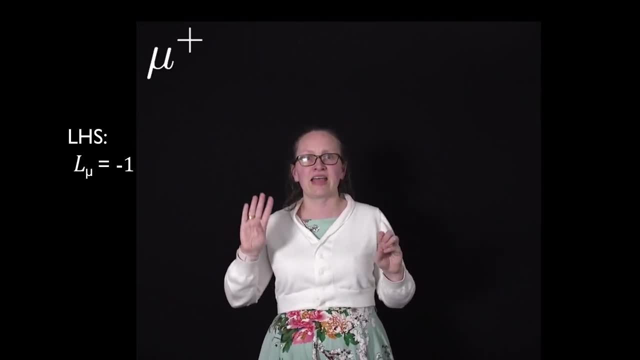 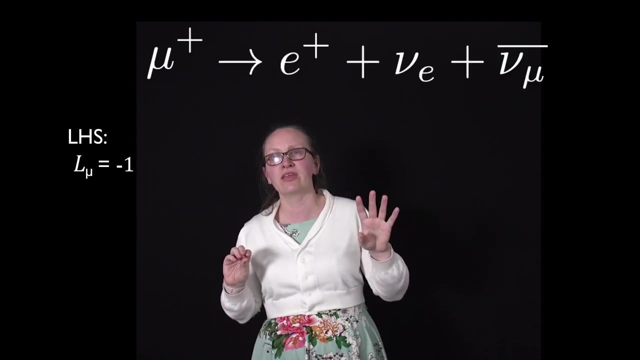 number. So let's consider an example of a case where this holds. We can consider the decay of an anti muon. So an anti muon has a muon lepton number equal to negative one. When it decays, it decays into a positron, an electron neutrino and 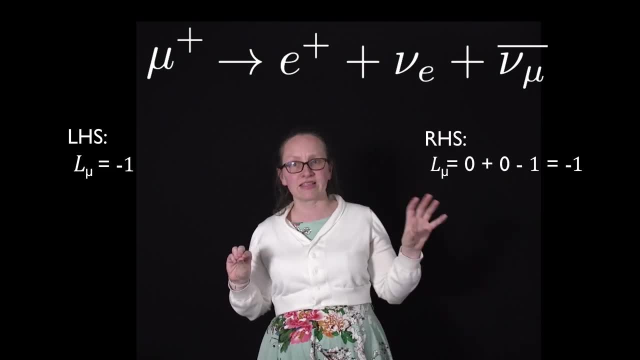 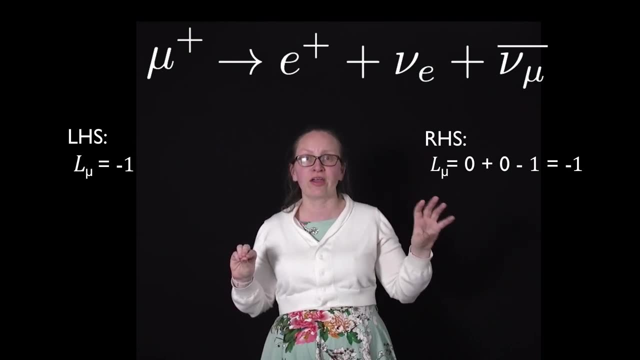 an anti muon neutrino. So on the right hand side the only one of those particles with a muon lepton number is the anti muon neutrino And this has a muon lepton number equal to negative one. So you can see on the 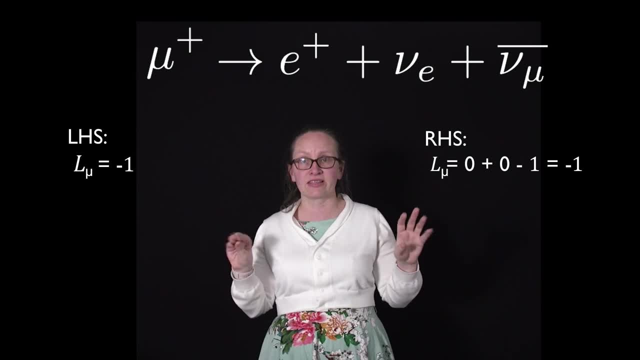 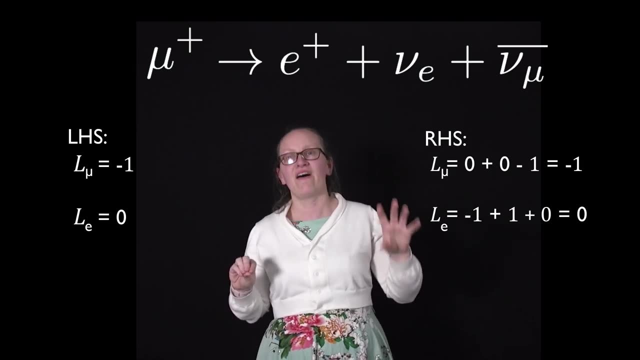 two sides the muon lepton numbers are balanced. Now, on the right hand side, we also have a positron with an electron lepton number of minus one and an electron neutrino with an electron lepton number of plus one formed. So the electron lepton numbers on both sides of the equation are also equal to zero. So 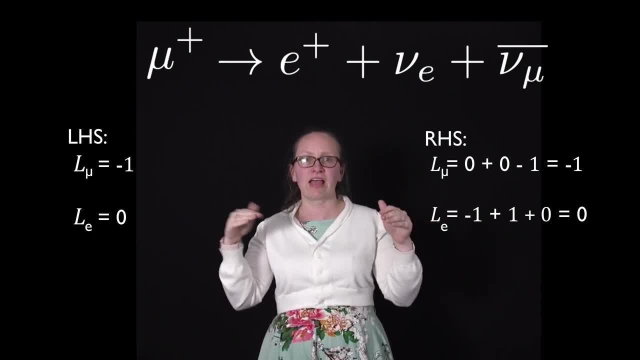 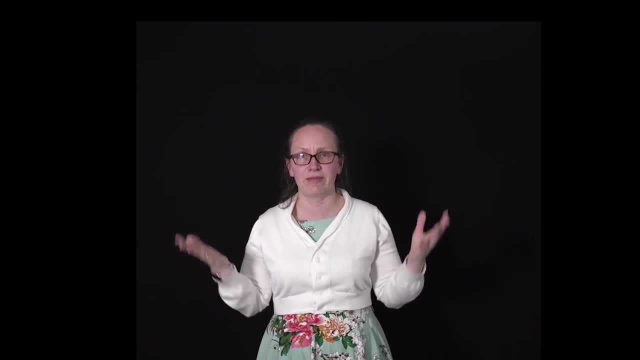 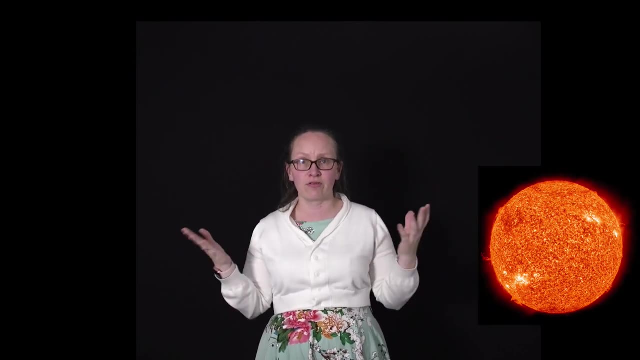 in almost all cases the different flavours of lepton number are also conserved. but this understanding led us to a bit of a puzzle. We know that electron neutrinos are produced in the Sun, so one example of a reaction producing electron neutrinos in the Sun is we can have two protons combining to. 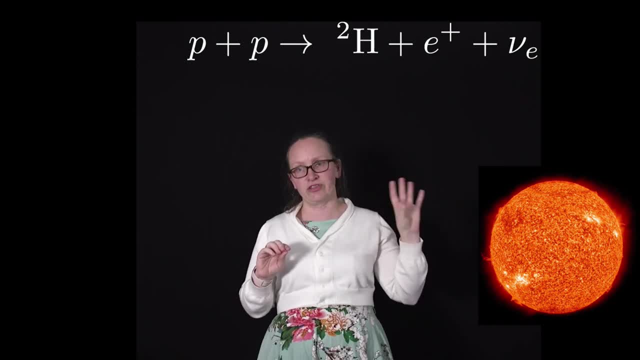 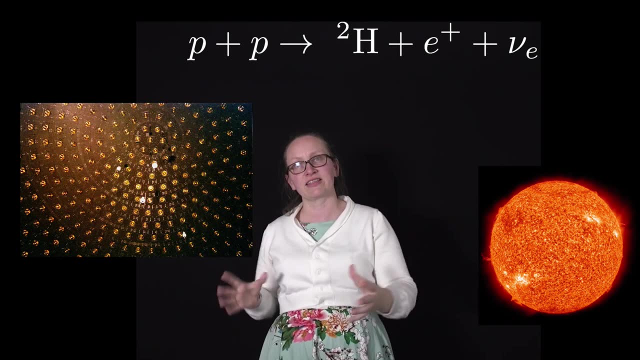 form deuterium, a positron and an electron neutrino. So these electron neutrinos travel from the Sun to the Earth to form neutrinos. So these electron neutrinos travel from the Sun to the Earth, to the Earth, sun towards the earth. and with special apparatuses involving large tanks of deuterium, we can actually 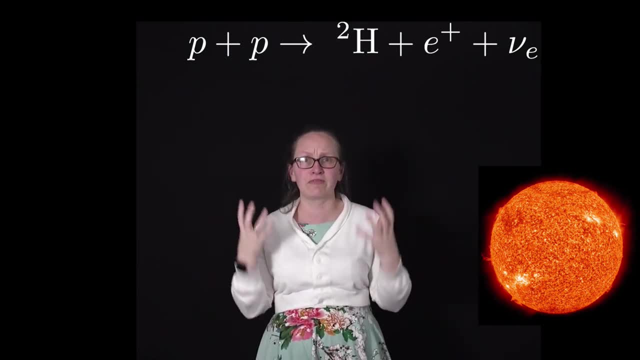 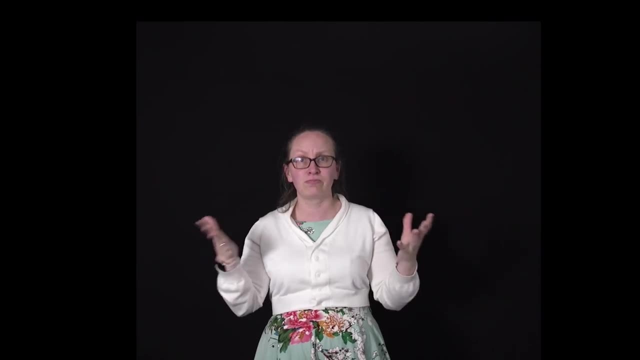 detect them, And for a long time people were very puzzled because we were only detecting approximately a third as many solar neutrinos as we expected. So at that time it was thought that neutrinos had no mass. So it turns out that in fact, this conservation law for the different flavours of leptons